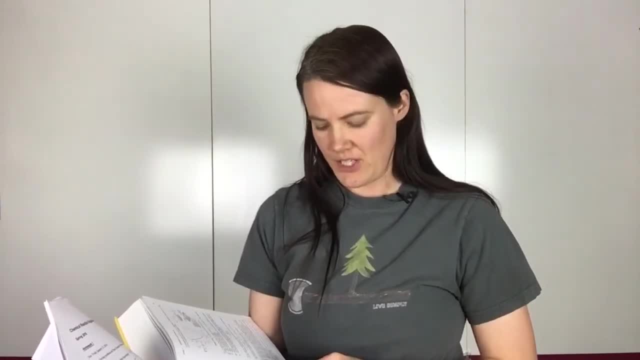 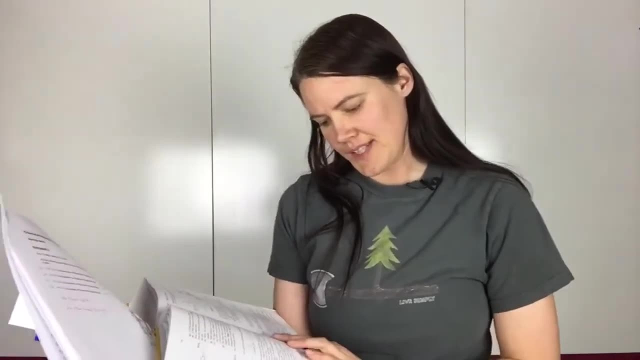 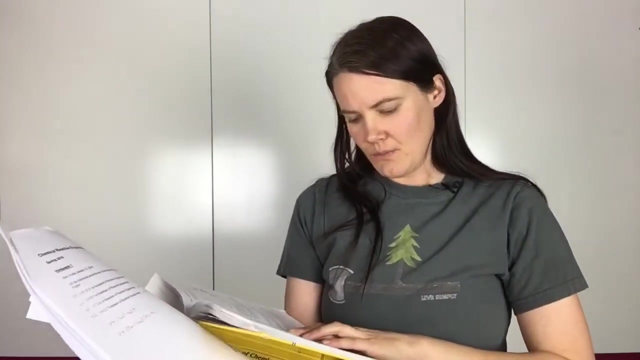 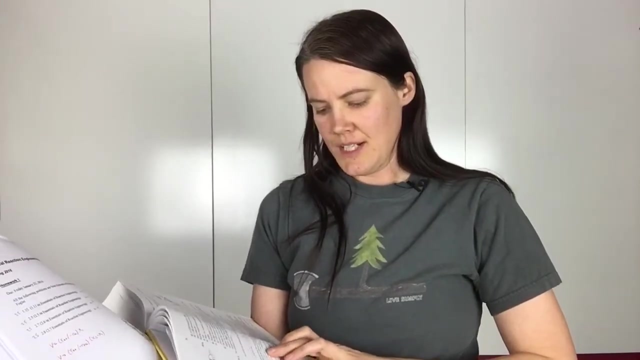 And then it gives you some data for X, the conversion and the rate that they recorded for each conversion. And then it has a few parts. The entering molar flow rate of A was 300 moles per minute. And then for part A it says: what are the PFR and CSTR volumes necessary to achieve a 40% conversion? B- over what range of conversions would the CSTR and PFR reactor volumes be identical? 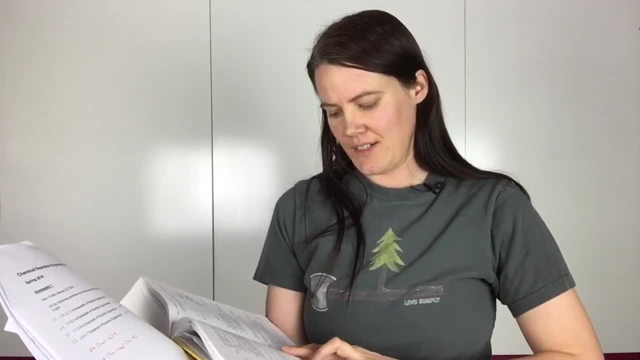 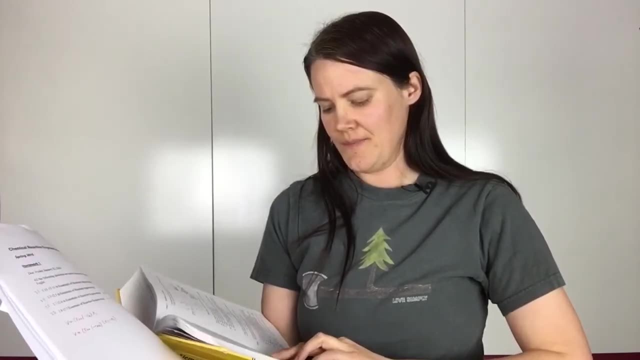 C. what is the maximum conversion that can be achieved in a 105 dm cubed CSTR? D- what conversion can be achieved in a 72 dm cubed PFR that is followed in series by a 24 dm cubed CSTR? 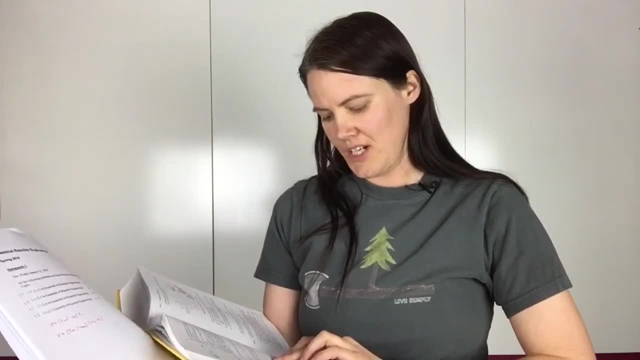 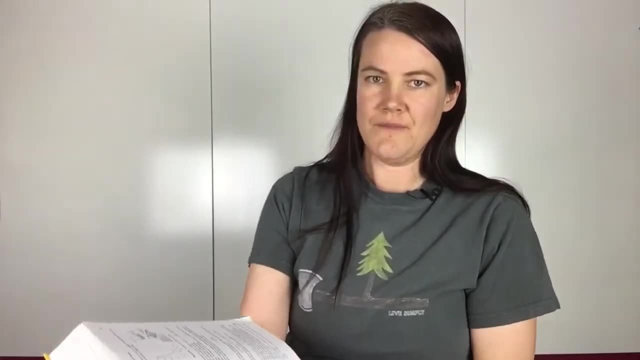 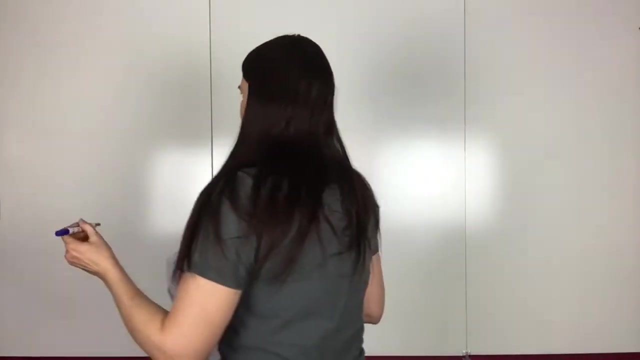 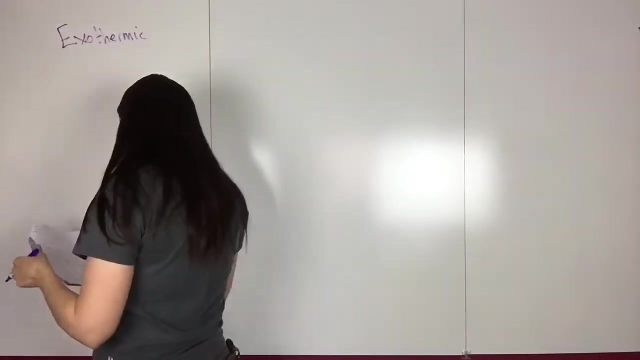 And then for part E, what conversion can be achieved if a 24 dm cubed CSTR is followed in a series by a 72 dm cubed PFR. So I'll just go ahead and start writing some of this stuff down. First of all, it says that it's exothermic. It's A to B plus C. 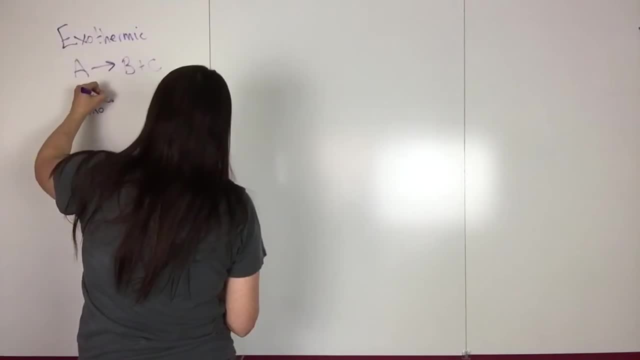 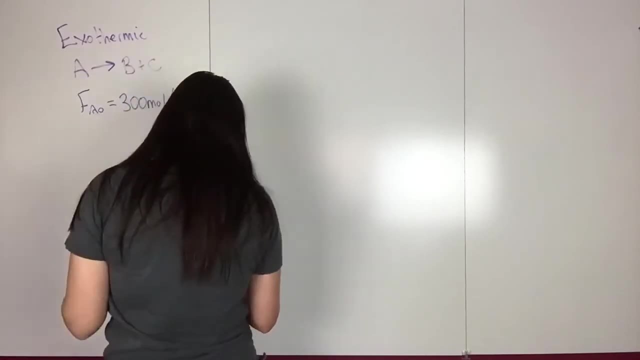 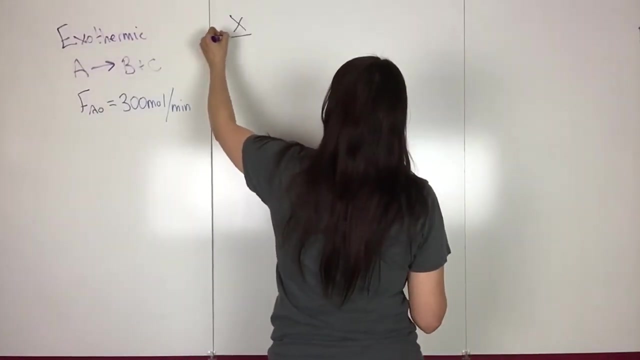 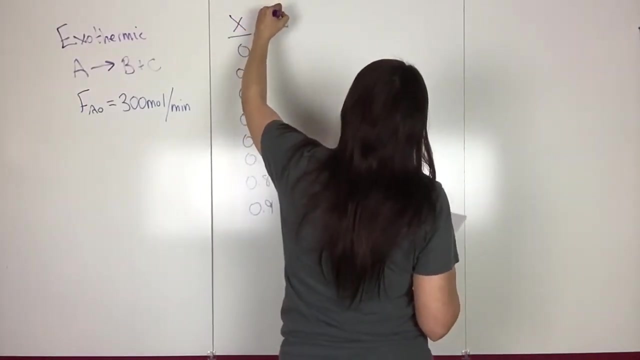 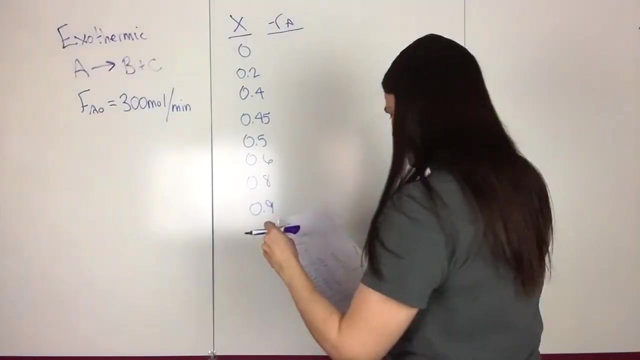 You know that FA0 is equal to 300.. Moles per minute. And then it gives you the following data: X, So 0, 0.. These are the conversions And then. so this would be what you would have if you were, say, running an experiment and measuring data. 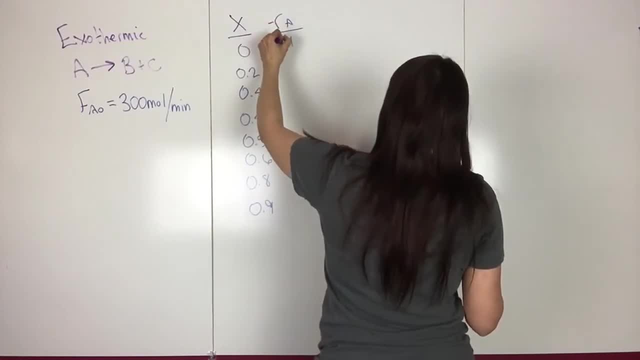 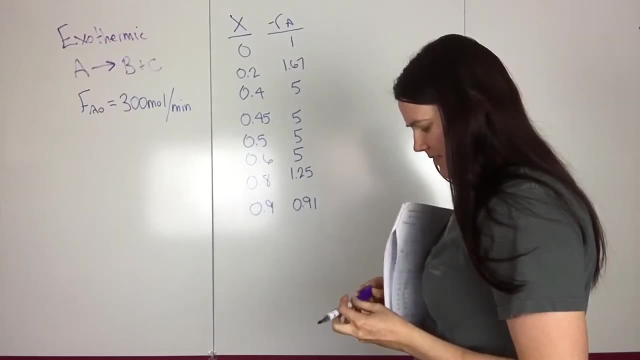 So then, for the rates for each of these conversions, you had 1.. So this is the data it gave you, And the easiest way to solve this problem is going to be from a plot. So we want to make that. we want to make a plot. 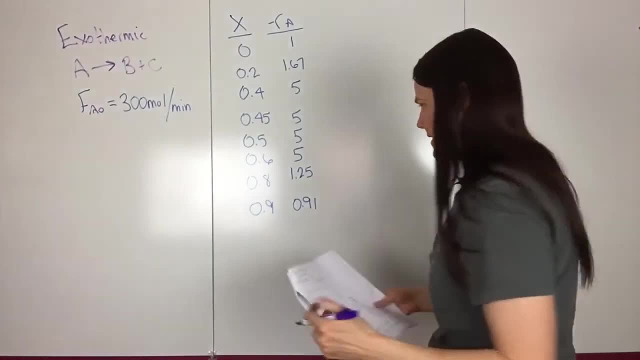 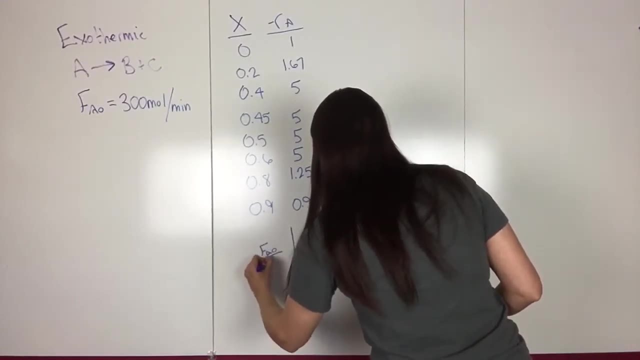 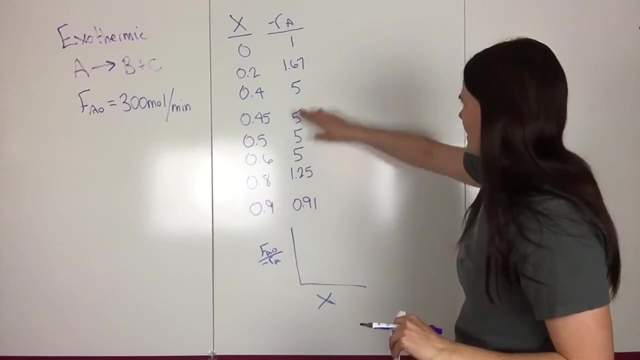 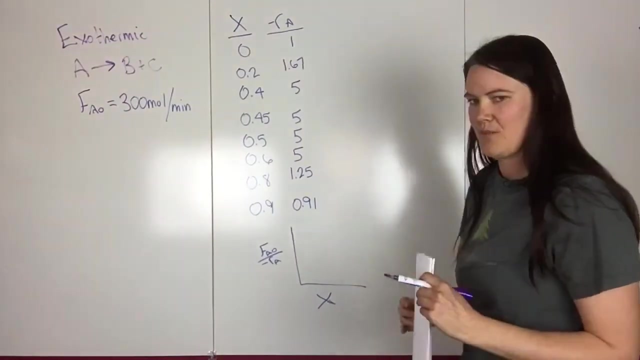 And the plot we want is going to be something like this: So the FA0 over minus RA to X. So we have everything we need for that, So we want. so the way I usually do this is: I'll make another column with the whatever I'm plotting. 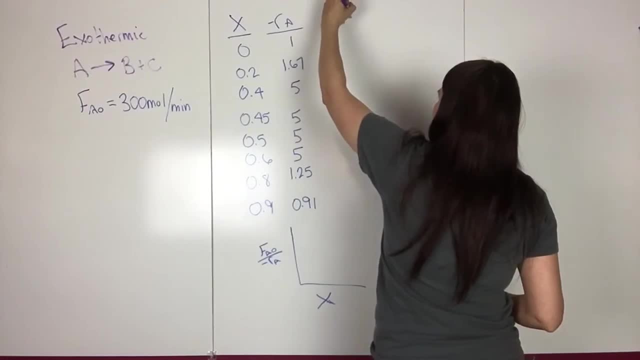 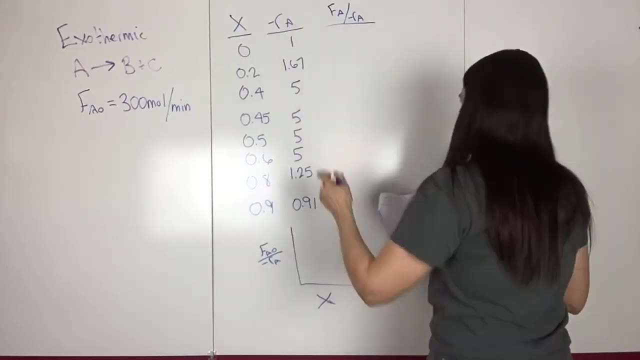 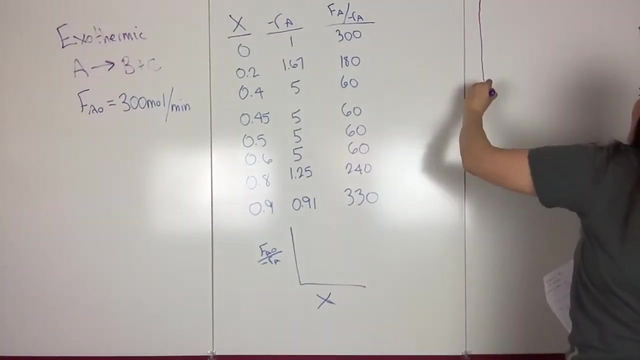 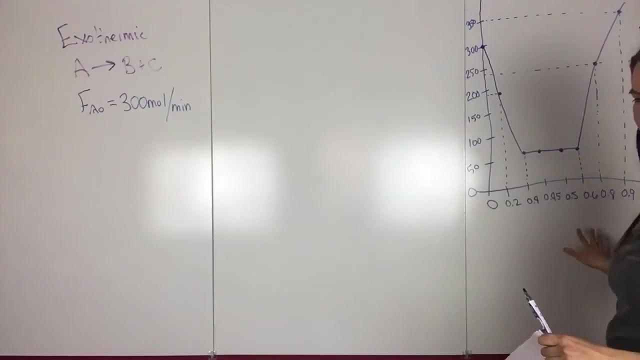 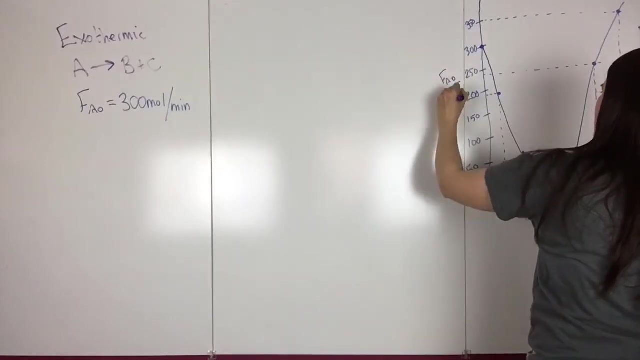 So FA0 over RA, And we know what FA0 is, so I just went through and calculated all these, So this one's 3.. And then we want to go ahead and plot this. So this is the plot we get. and oh yeah, so this is FA0 over minus RAX. 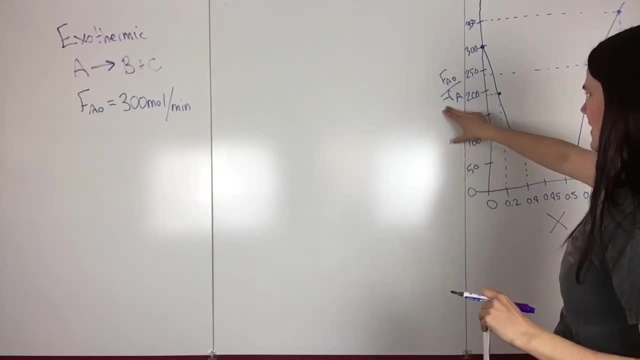 You want to be careful with these, because sometimes only 1 over RA is plotted by X, And so then to get the volume. so the way I have this plotted here, to get the volume, it's just the this multiplied by this. But 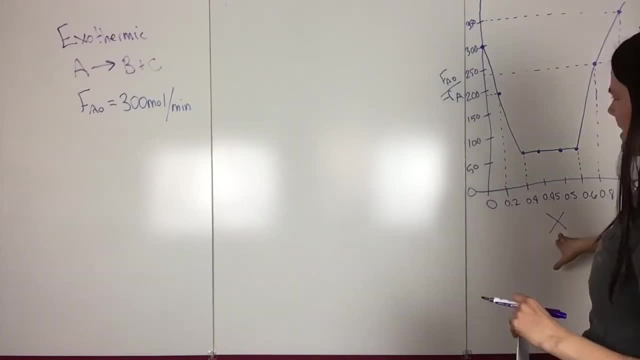 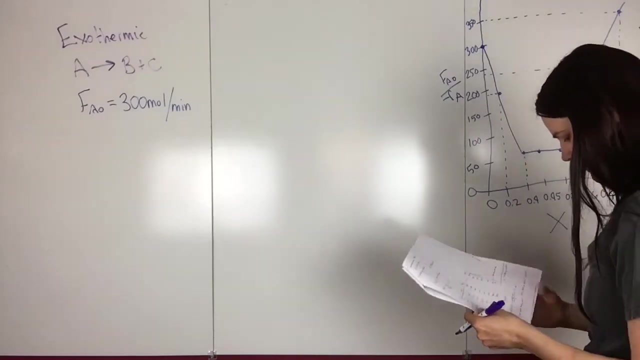 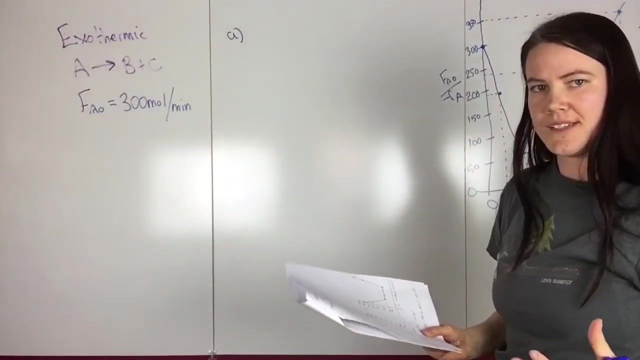 if you for a CSTR anyway. but sometimes the plot will just be 1 over the rate by X, And so then you would need to also multiply everything by FA0.. So just keep that in mind. So for A, it's asking for the volume of a CSTR and also a PFR. 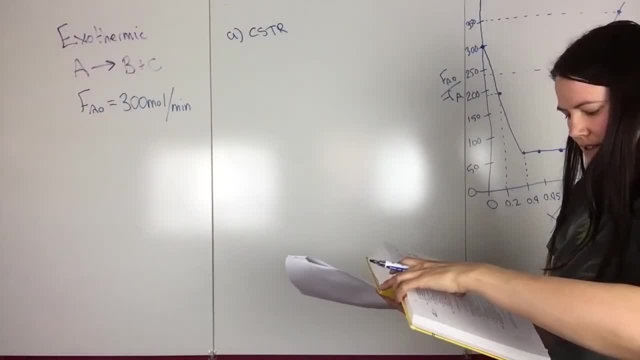 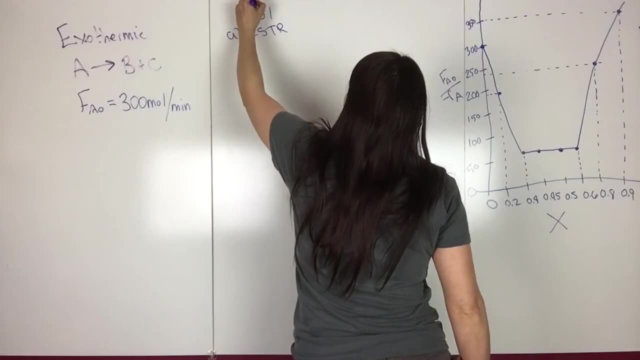 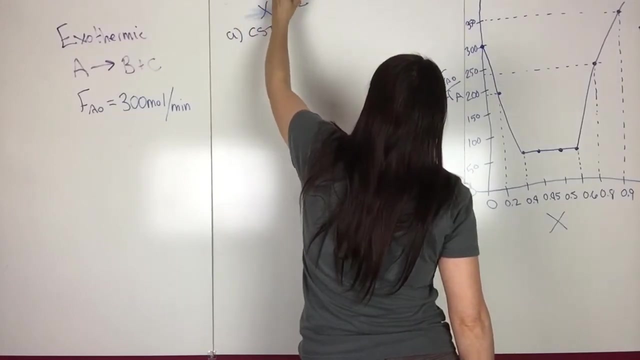 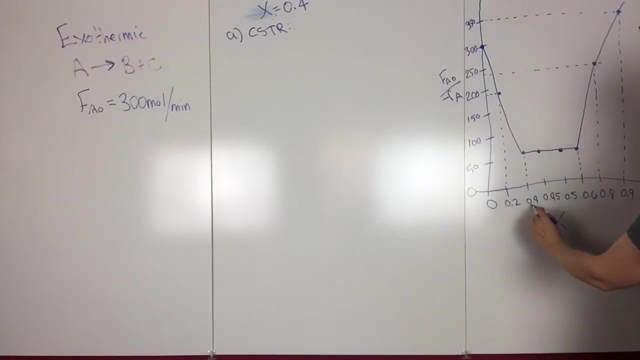 So it's asking for the PFR and CSTR. So it's asking for the volume necessary for 40% conversion. so 40, oh, I'll write that different X equals 0.4.. So for a CSTR we can just go to this plot, and X equals 0.4 is right here. so then we would just draw up and over. 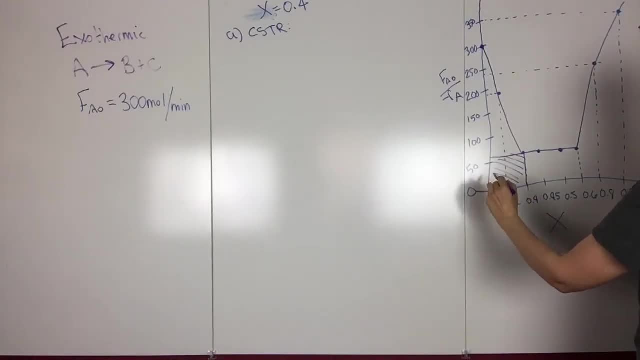 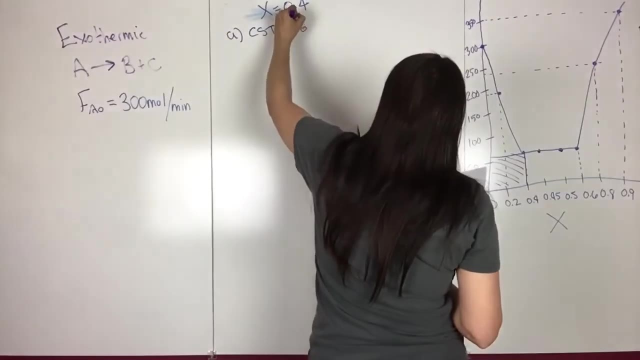 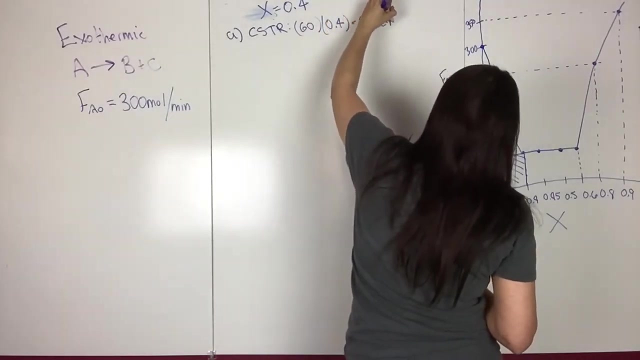 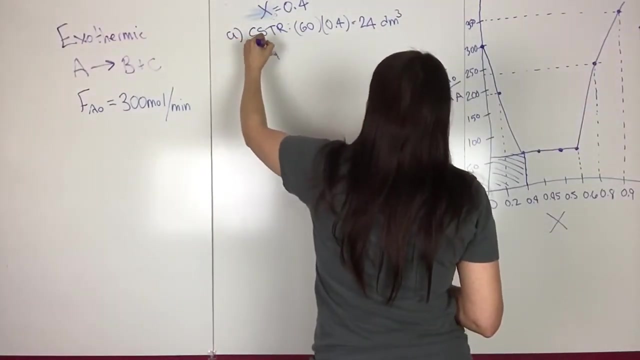 And then it's just this area. So that was well, and I guess that's about 60.. So 60 times 0.4, and that's equal to 24 DM cubed. So then, for the PFR at 40%, it's the error. 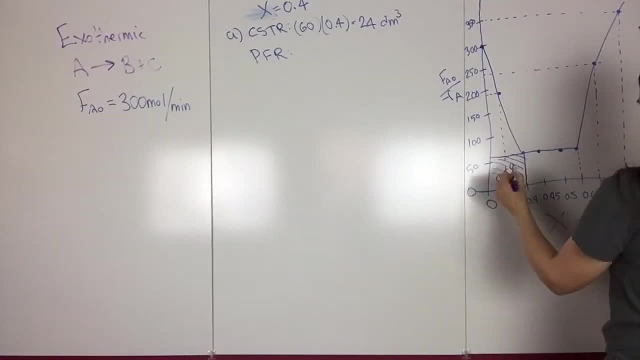 So this is the CSTR And for the PFR we go over to 40% or 0.4.. And then for the PFR it's this entire area, because it's the area under the curve. So we just need to add all that up. 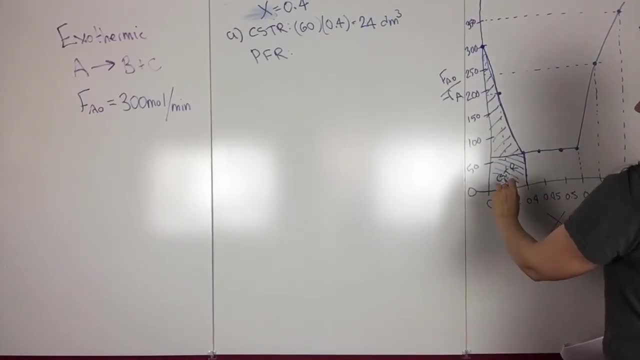 And we just need to calculate this area. So the way I did it was I just took. so we already have the area under the curve, So we already calculated the area for that part. So it's just the 60 multiplied by 0.4 plus. 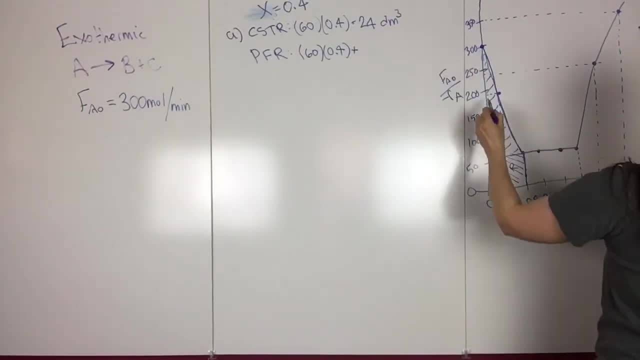 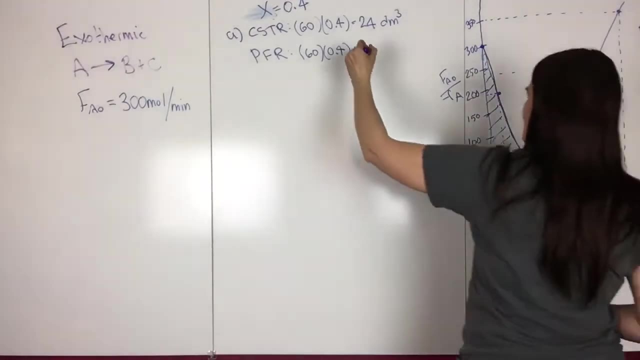 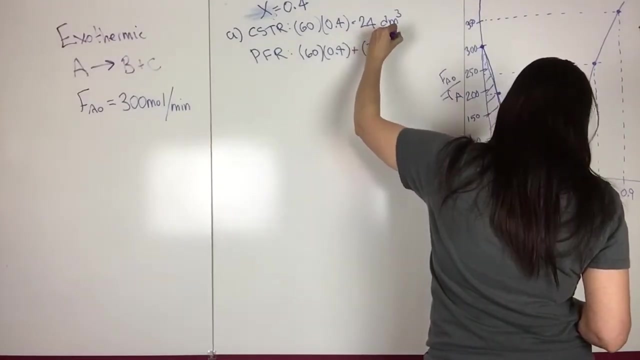 and then we want the area under this curve And I just said, okay, 300 minus 60 multiplied by the 0.4.. And then we need to divide that by two, because this is just half of that rectangle. So 300 minus 60 multiplied by 0.4.. 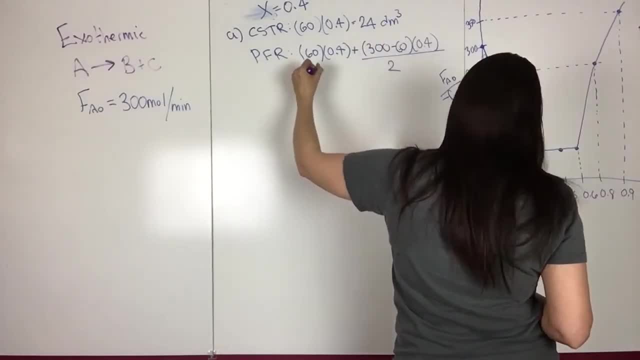 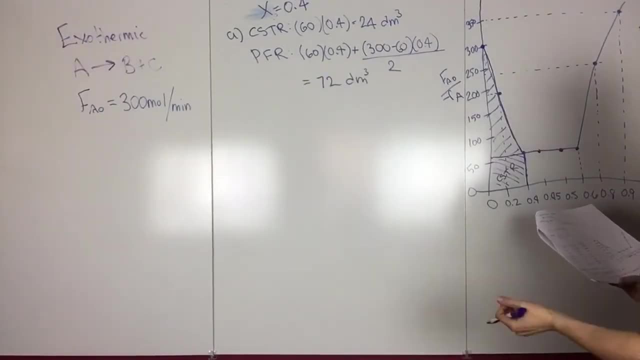 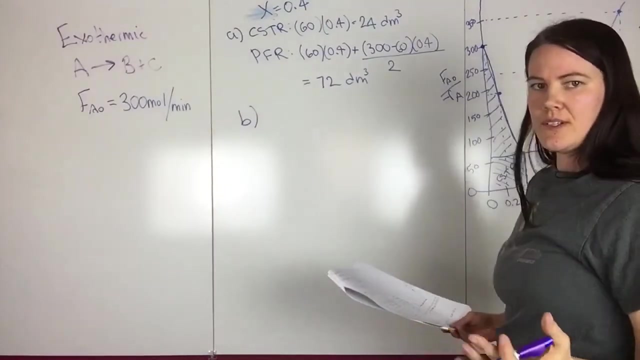 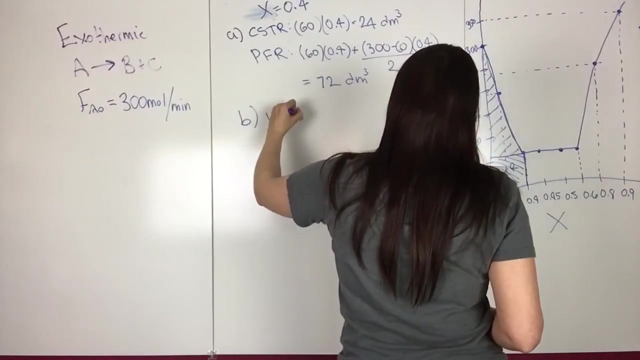 0.4 divided by two, and that's equal to 72 DM cubed. And then, for B, it wants to know over what range would the volumes of the CSTR and the PFR be identical? So volume of PFR and CSTR. 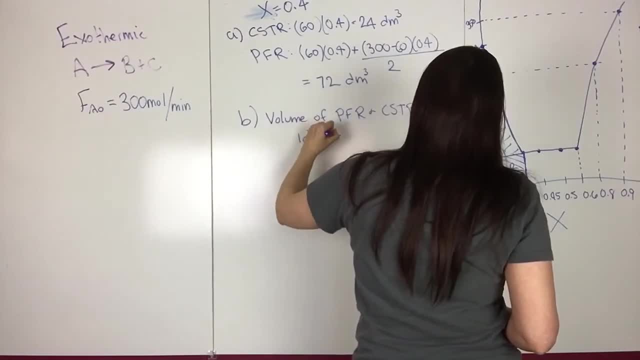 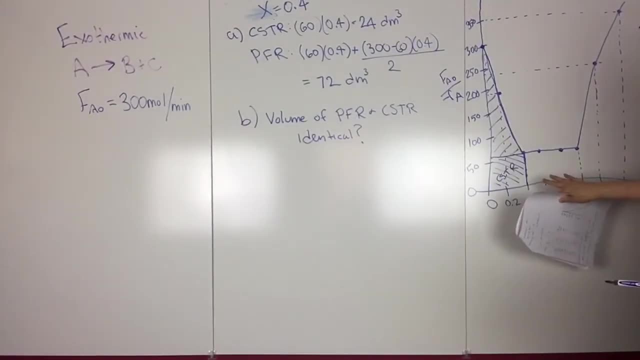 Identical. So if we look at this graph, we know that for the PFR, the volume is the area under the curve And we know that for the CSTR, it's the area of whatever square or rectangle you end up making, based on where you end up on this plot. 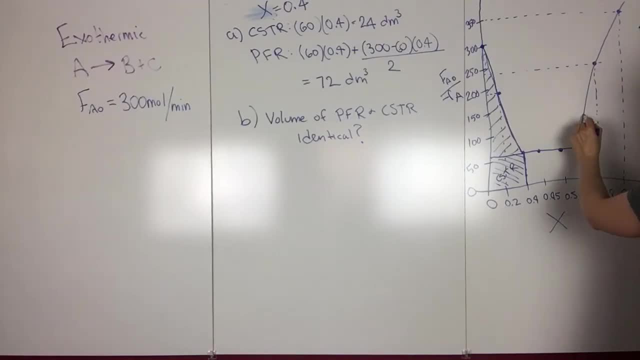 So, for instance, say you are at 0.6.. 0.7, and then you go up to here. for the CSTR it would be this entire area here And that would be the volume, And for a PFR it would be just this area under the curve. 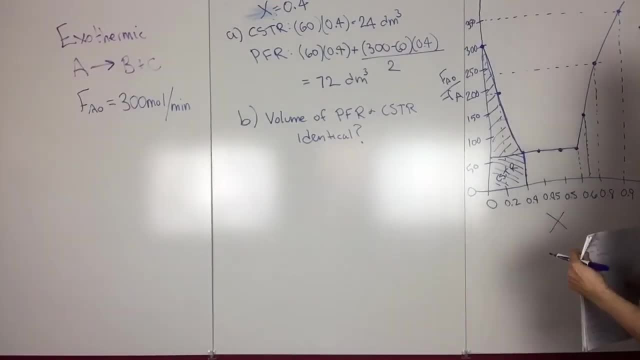 So then, looking at this, it's pretty, we can see that they'll be identical. So then, looking at this, it's pretty, we can see that they'll be identical. So then, looking at this, it's pretty, we can see that they'll be identical. 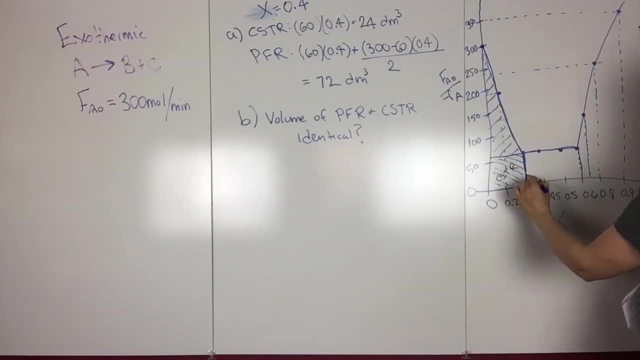 Right here. And the reason why is because, if we have, and just so, from the 0.4 to 0.6, not from 0 to 0.6.. So from 0.4 to 0.6, the area, the CSTR. 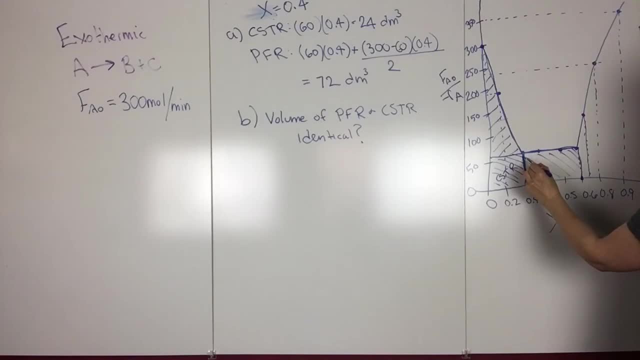 So if we go up from 0.6, then the CSTR is this area And then for the PFR it's the area under the curve, So they're identical volumes, And then for the PFR it's the area under the curve. 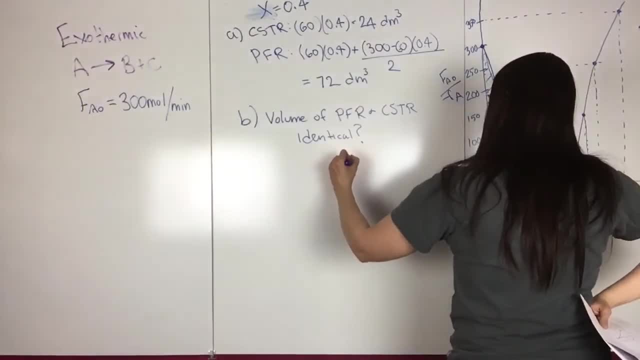 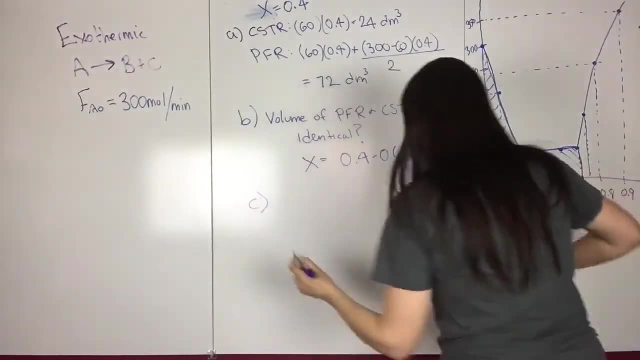 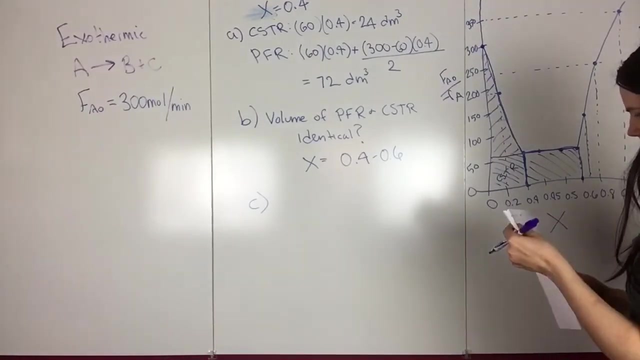 So these are identical volumes from 0.4 to 0.6.. So for CSTR, it wants to know, all right, or it stays that your volume, So volume is one, partnering for volume, All right. So again, these are identical. 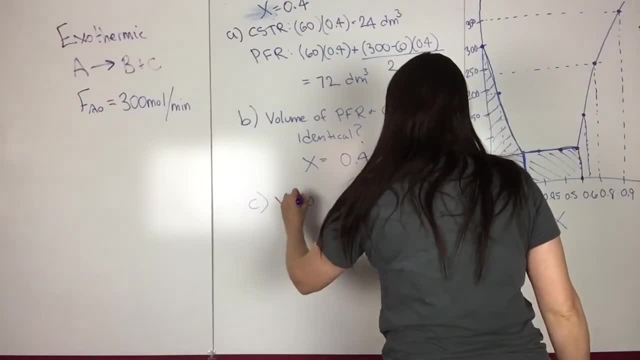 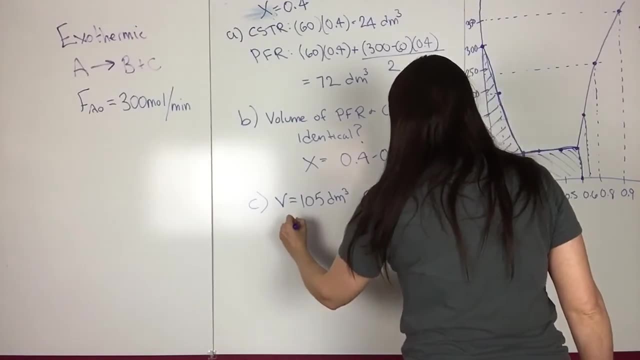 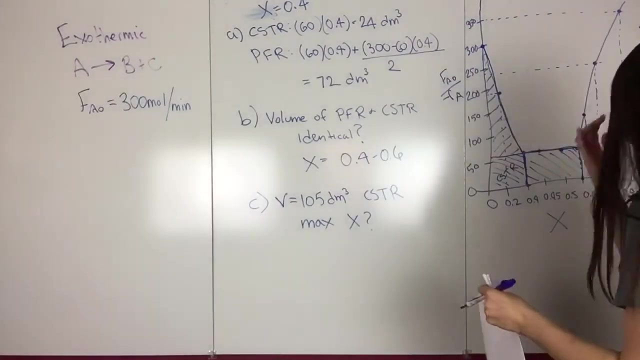 We just have a quantity here. We have a number in here here. Now we're going to call it volume, Because these are identical volumes: 105 dm cubed in a CSTR, and it wants to know what your maximum conversion is. 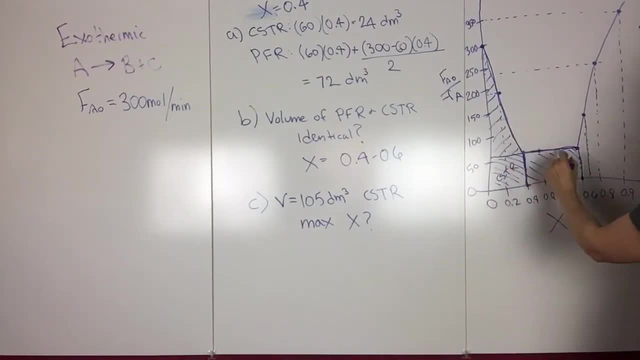 So the way you can solve this is just looking at different points on this curve. So this is kind of trial and error. So let's say, maybe you think it's 0.6.. So if you go up, 0.6 is right here. 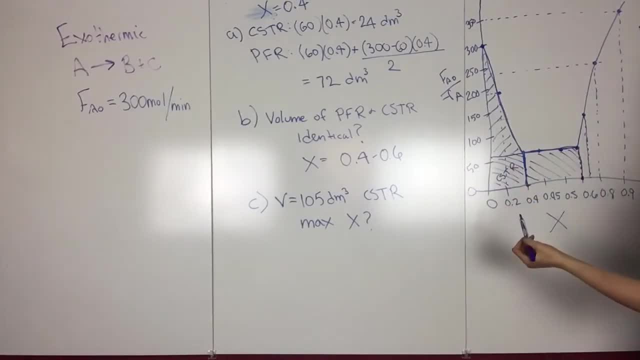 So 0.6 times 60, so that would have a volume of 36 dm cubed. So you know that it has to be higher than 0.6.. So if you go up to say 0.8, 0.8 times about 240.. 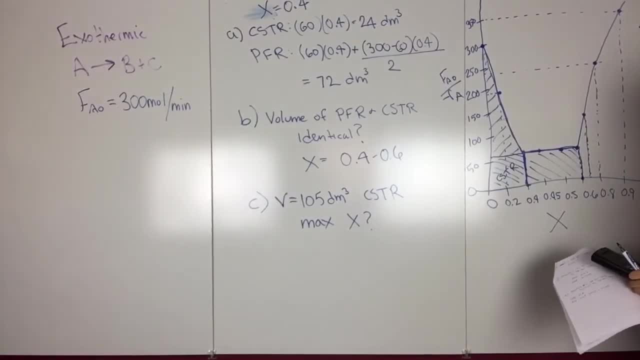 So 0.6.. 0.8 is 192, so you know it has to be less than that. So maybe try 0.7.. So 0.7 multiplied by looks like about 140, and that's 98. So it's somewhere around 0.7.. 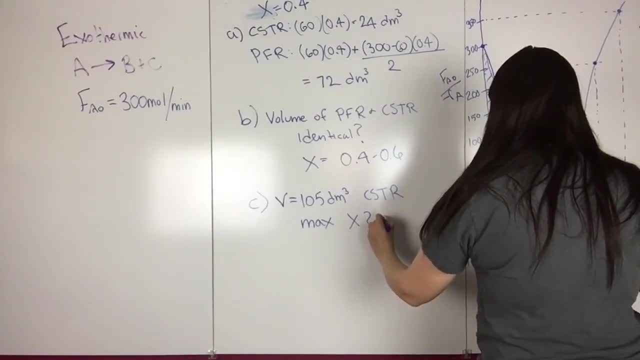 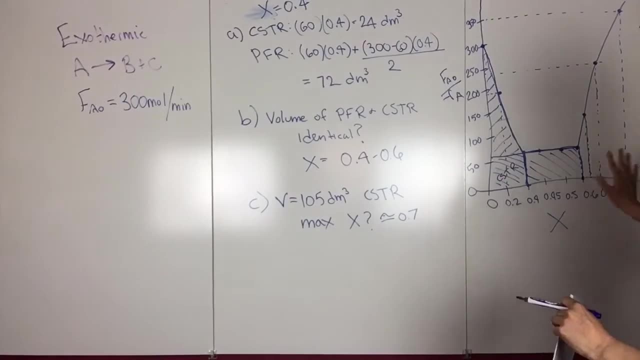 So x. So the max is: So x is approximately 0.7, and you could probably get more exact than that, but for this I'm not going to worry about it. So for d it says: alright, I'm going to erase some stuff off this plot real quick. 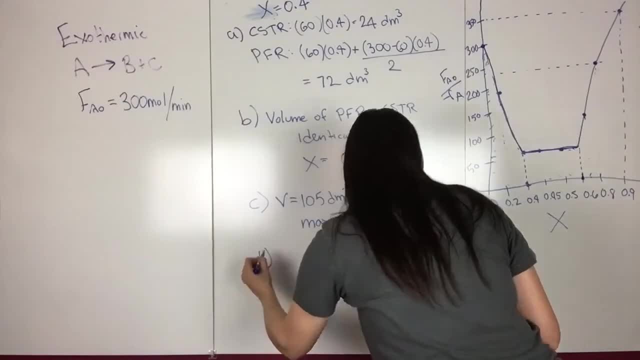 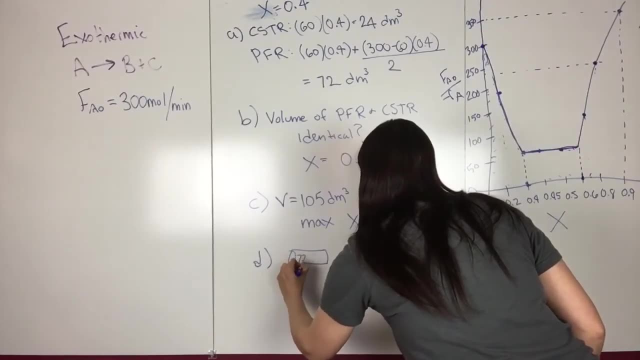 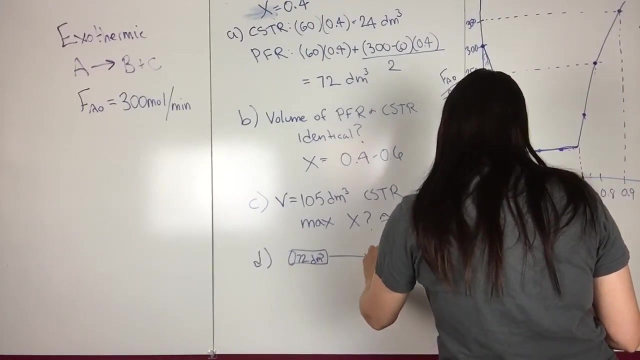 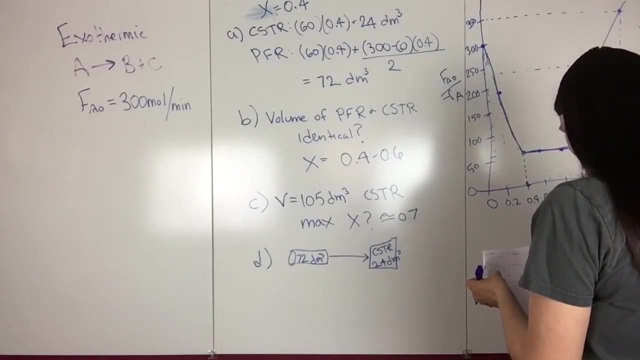 So for d it says you have 72. You have a PFR that's 72. Dm cubed and that's followed by a CSTR that's 24 dm cubed, and it wants to know. it wants to know what the conversion of these are. 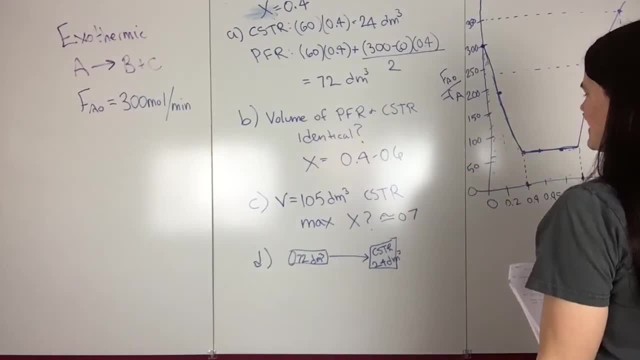 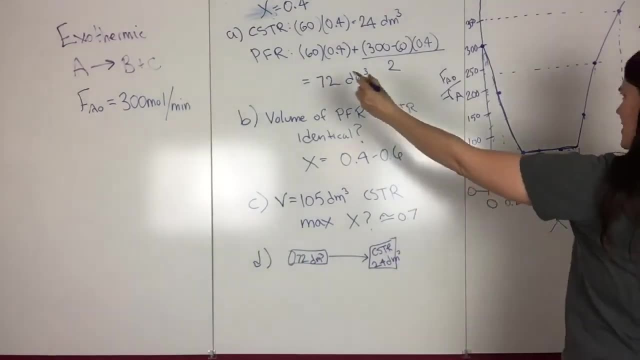 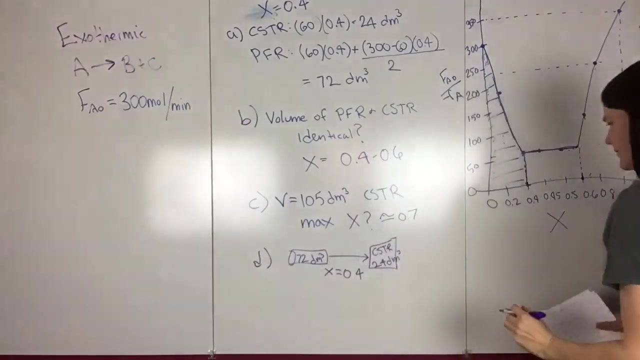 So we already know That the PFR for 72, we already know the conversion for a 72 dm cubed PFR was 0.4 because we calculated that in part a. So we know that this is the PFR and we know that x is equal to 0.4.. 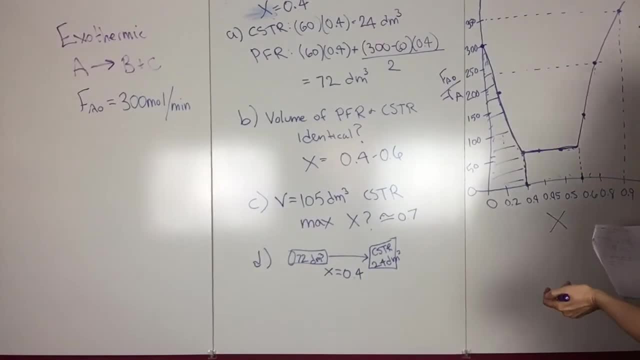 And then for the CSTR, We, We, We Kind of need to do this trial and error thing again where we figure out: okay, well, where on this curve does Where From 0.4.. To somewhere along here, multiplied by something over here, that equals 24.. 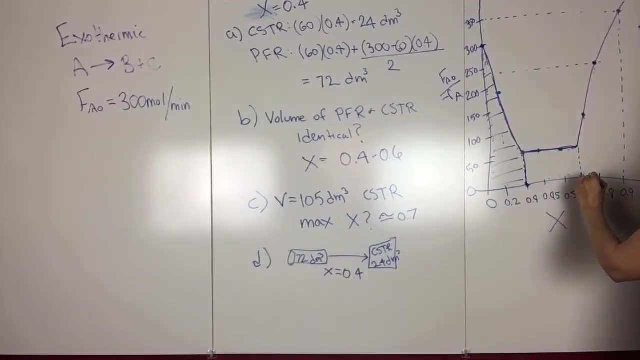 So it turns out the answer is around 0.65, and once again you would kind of arrive at through trial and error, but your PFR volume would look like this, or I mean, sorry, your CSTR would look something like this, and then this was: X equals 0.65, and then for part E it's kind of similar to D. 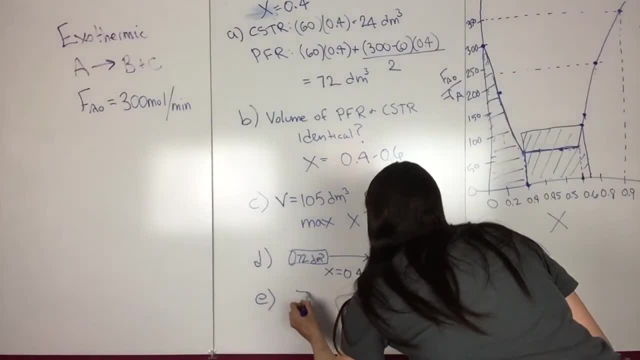 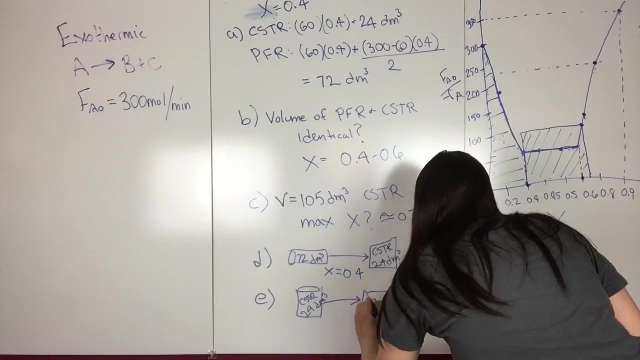 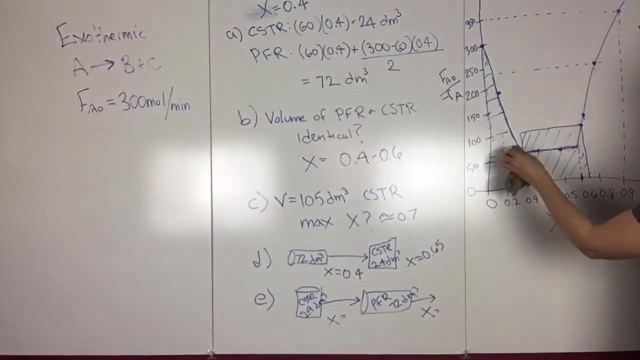 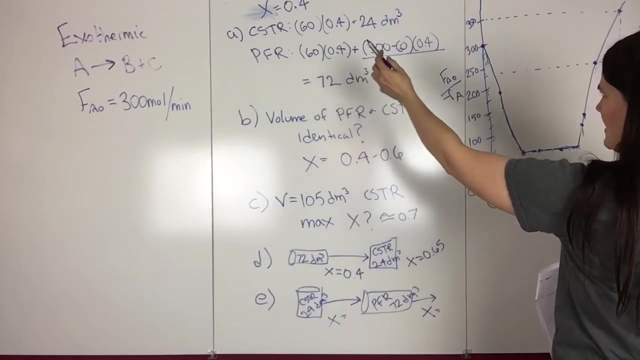 only this time you have a, you have the 24 DM cube CSTR followed by the 72 DM cube PFR, and it wants to know these conversions again. I'm going to erase this real quick. So we already know that the 24 DM cube CSTR is point four, because we calculated 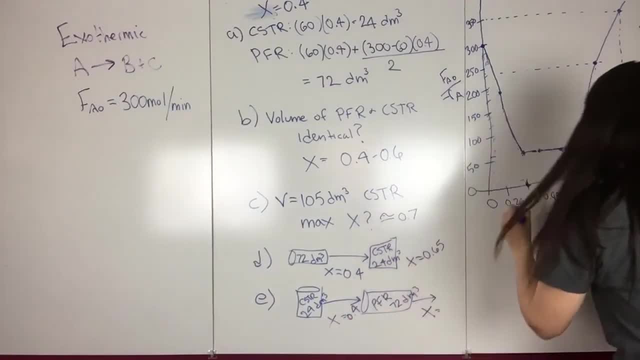 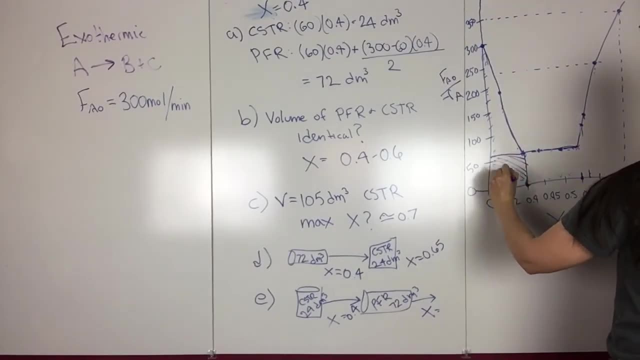 that. so x equals zero point four for that one and this looks like this, and then for the PFR. it's once again trial and error. so just try again and keep going and add something into this error. we need to figure out where under the curve, so somewhere from here over to 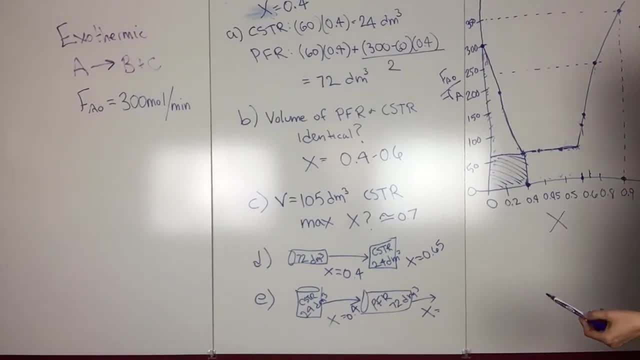 somewhere along here, and I already know the answer is around 0.9. but just normally this would be trial and error, like the previous problem I went through, so you would maybe try to go along here, maybe try 0.6, 0.8, and so anyway, what? 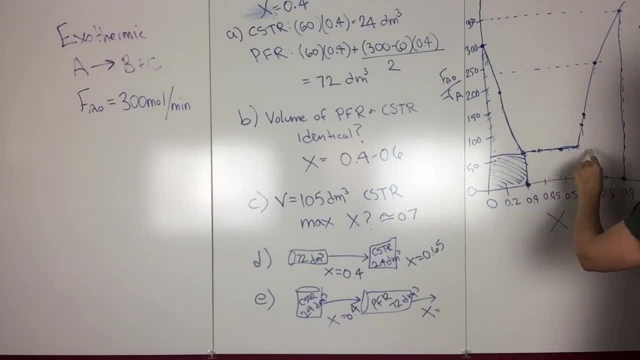 you're doing is once again just adding up this area under the curve. so you just need to find where the area under this curve is equal to the 72 DM cube. so kind of a takeaway for these graph problems is learning to recognize the difference between what a CSTR looks like on the 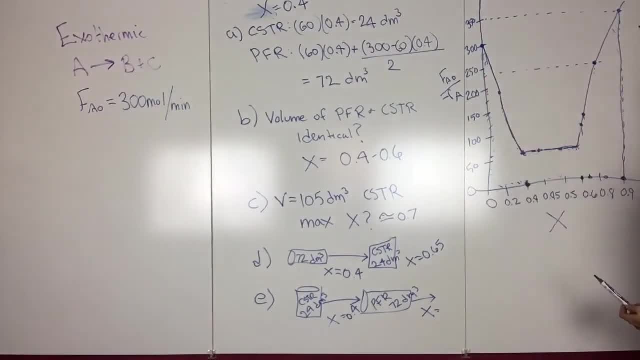 plot and what a PFR looks like. so just always remember that the that the PFR is the area under the curve and the CSTR is whatever area you get to. so like say, for instance, your cstr has a 0.5 conversion, then it would be this: